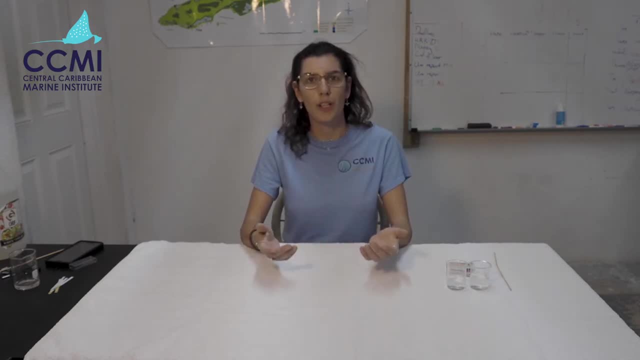 decrease in the pH of the ocean. Now I know that pH can actually be quite a confusing thing to explain to some of the younger students, so I'm just going to quickly go through how I explain it in my classes and hopefully that will give you a little bit of help. 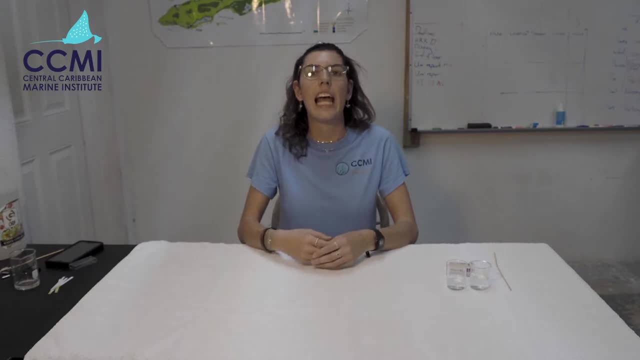 in that area. So pH is actually a scale and pH stands for the potential of hydrogen. Now, all solutions are normally acidic or they are alkaline and they fall somewhere on this scale. Acids have lots of hydrogen ions inside of them and alkalines do not have very many hydrogen ions. 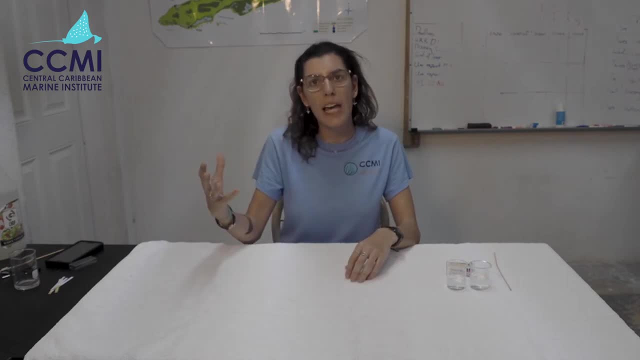 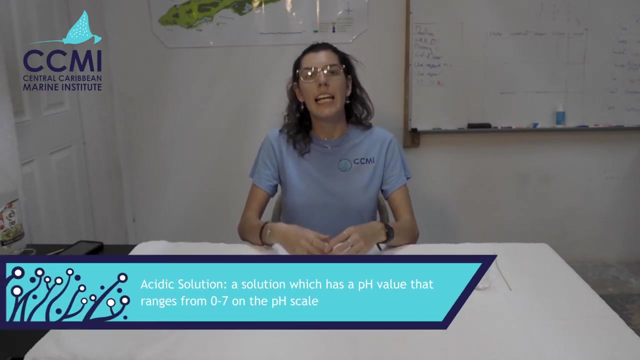 inside of them, Alkalines have a high pH and acids have a low pH. So this scale runs from 0 to 14.. If the pH is less than 7, then it means that it is an acidic solution, and there are lots of those. 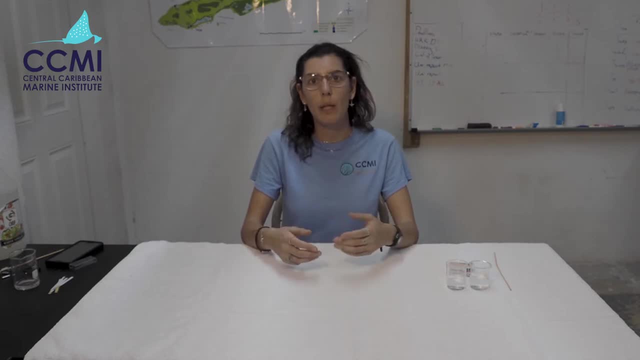 hydrogen ions inside of it, and if you have an acid with a pH of 0 or 1, it means that it's a very strong acid. If the pH is higher than 7, then it means it is an alkaline solution, and if the pH is. 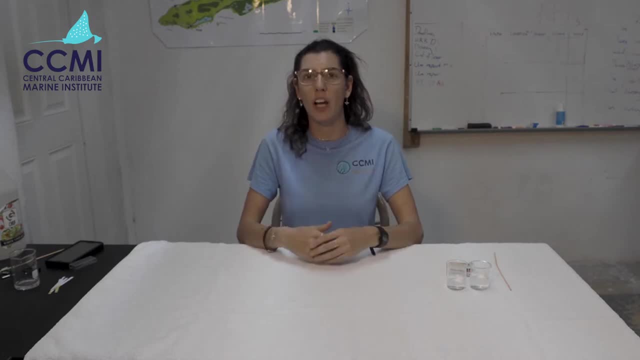 13 or 14, it means it's a very strong alkaline solution. If the pH is 7, then it means the solution is neutral and a common neutral solution that we find is pure water And they are not very reactive. Now going back to the pH of the ocean, 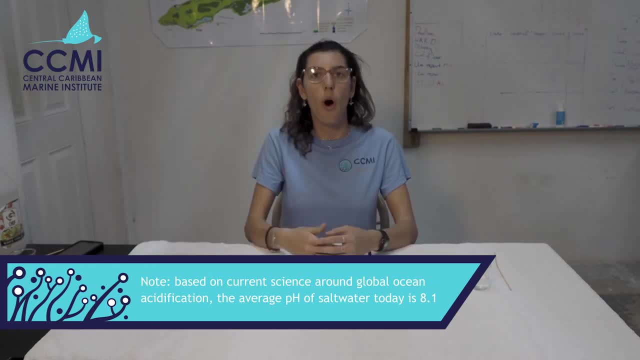 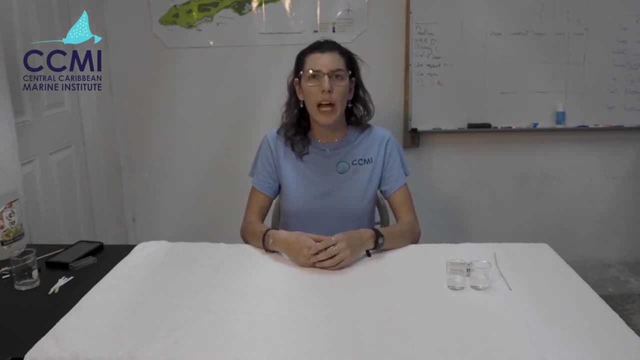 The pH of the ocean due to the absorption of this carbon dioxide has actually caused the pH of the ocean to drop from 8.2 to 8.1 in the last century. Now this doesn't sound like a very big decrease, but because the pH scale is a logarithmic scale, 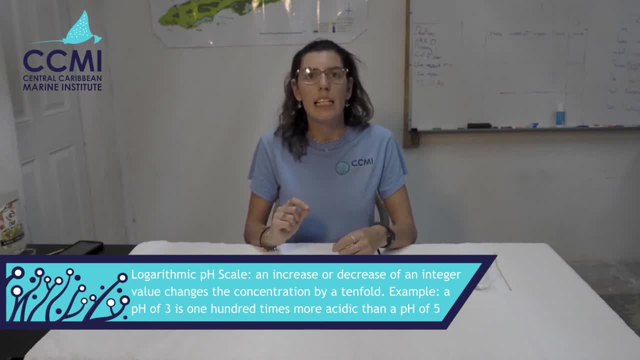 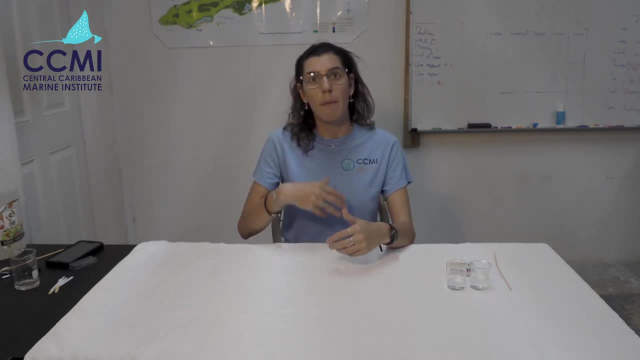 it does mean that this is actually a 20% decrease in the pH of the ocean, And if there continues to be the same amount of carbon dioxide put into the atmosphere as the current day, then they actually think that the pH may decrease a further 120%. which is going to have a huge impact on the life in the ocean. So what animals are going to be affected by this decrease? Well, it's mainly going to be the calcareous organisms that are going to be affected, such as the organisms with shells and, for example, the hard corals that form our coral reefs around. 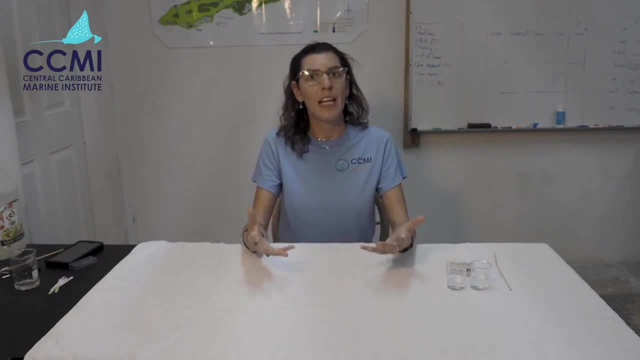 the island, Because what's going to happen is that when there is this increase in hydrogen ions in the sea water, there's much less carbonate ions, and they use these carbonate ions to actually form their shells and their skeletons. So if there's a decrease in hydrogen ions in the sea water, then 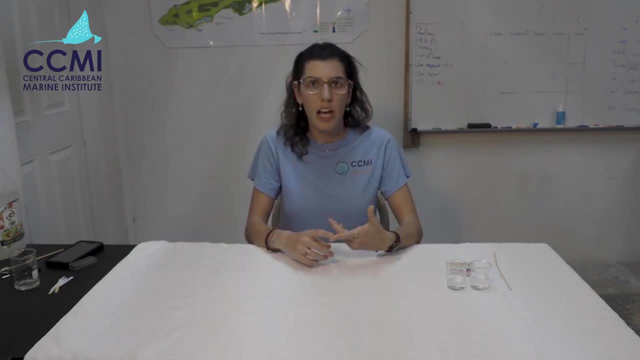 so by having less of these carbonate ions, the shells and the coral skeletons, they're, one, going to be harder to form and, two, they're actually going to be harder to maintain as well. So this is going to cause a really stressful environment for these creatures to live in. So it's really, really important that we actually try and reduce the amount. 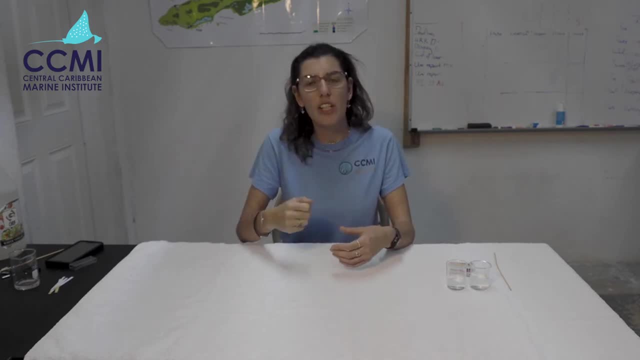 of carbon dioxide we're putting in the atmosphere and try to reduce down the amount of ocean acidification That is happening, because it can have a huge impact on the marine food web. Now, this is enough about actually what ocean acidification actually is. Let's get on and undertake the experiments that you guys were given the equipment for. 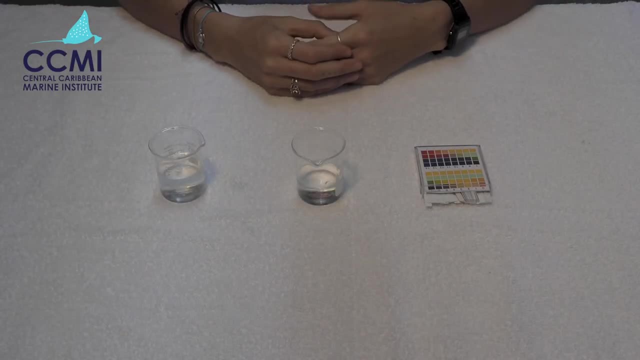 Okay, so let's go through and actually undertake the experiment. Now, this beaker right in front of me, I have actually filled up with seawater. Now, if you can't get to the ocean, you can't get to the ocean. Now, if you can't get to the ocean, you can't get to the ocean. Now, if you can't get to the ocean, you can't get to the ocean. 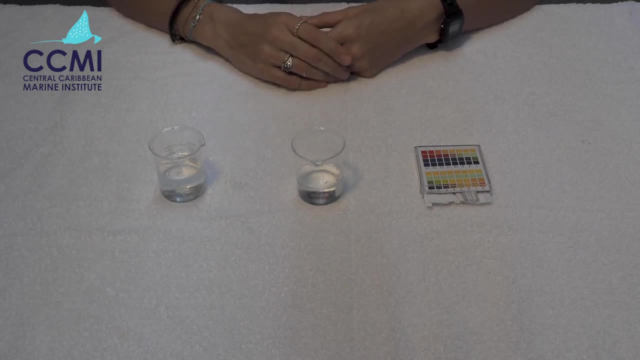 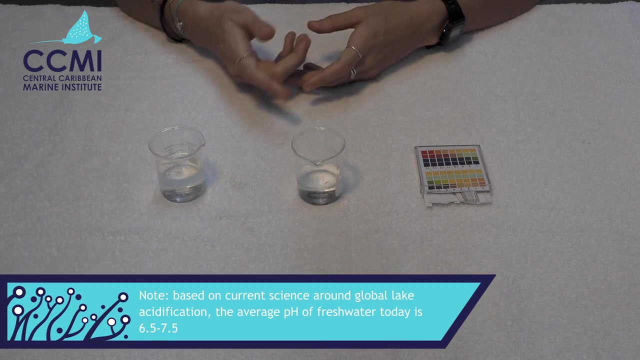 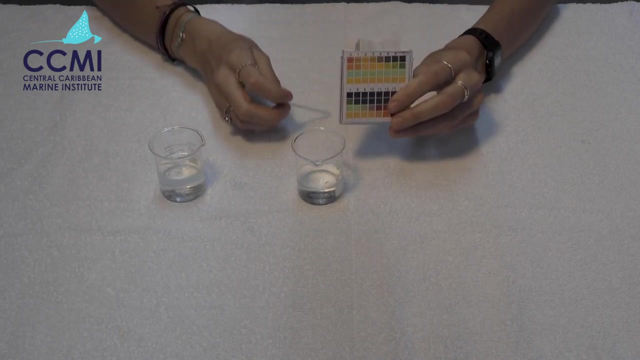 fill it up with seawater. that is not an issue. just fill it up with seawater from your tap. it is still going to have the same overall effect during this experiment. now what i'm going to do is i am going to take the ph test strips and, following the instructions on the front of the pack, i'm just 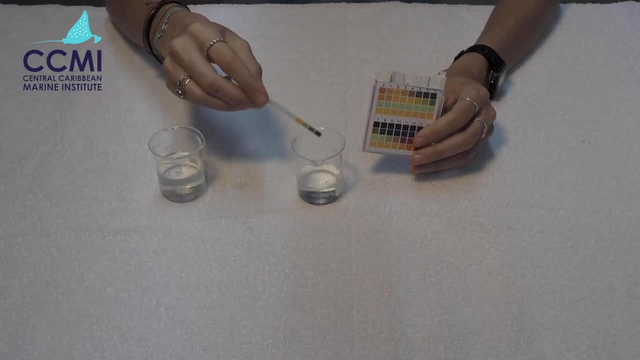 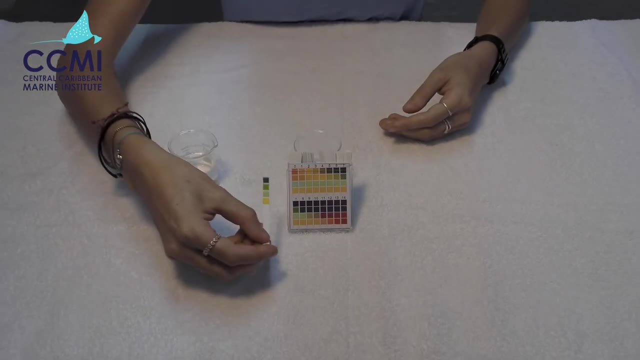 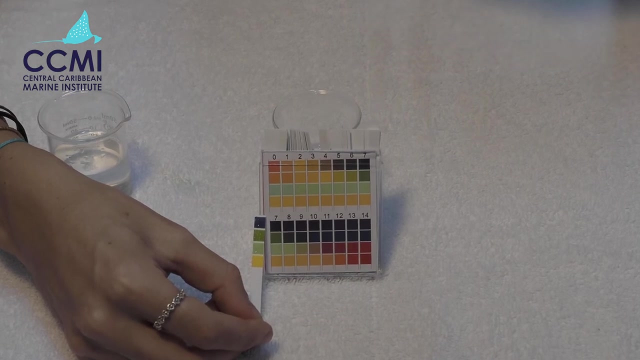 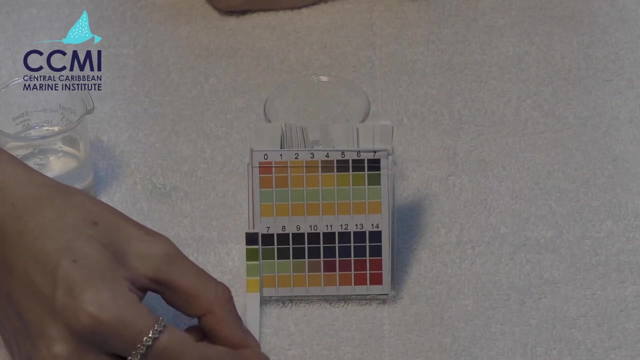 going to dip it in the water, take it out, and i'm going to knock off some of the excess water. now, if we look here, we can see that there are four different color strips, and what you're trying to do is you're trying to match those to the numbers that we are finding here on the back of the pack. if i hold mine, 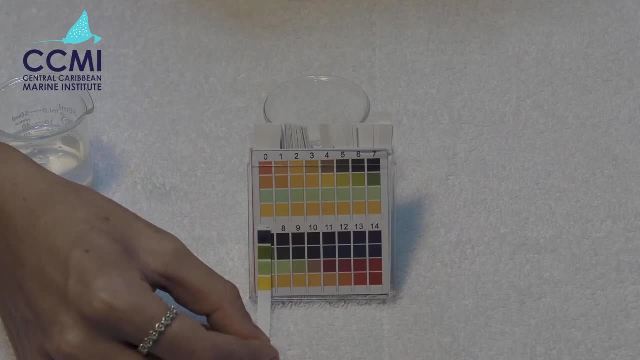 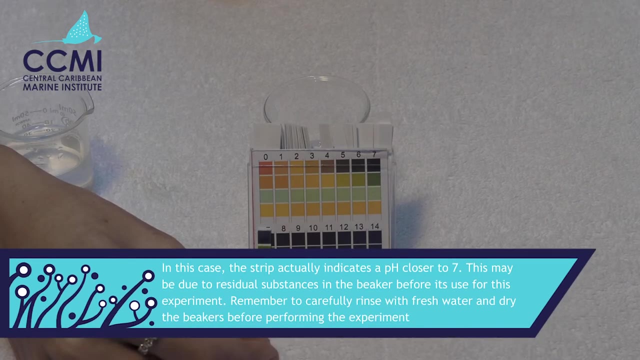 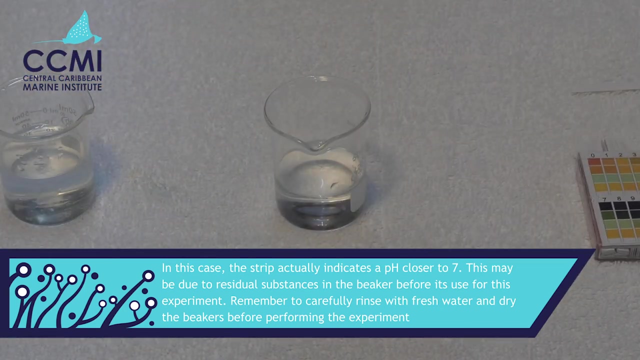 nice and closely. i think that mine are probably matching an eight, and that's because i took this seawater obviously out of the ocean and we know that it has a ph of around eight. so that is the first part of our experiment. now what we are going to do is we are going to add an acidic solution to this seawater in order 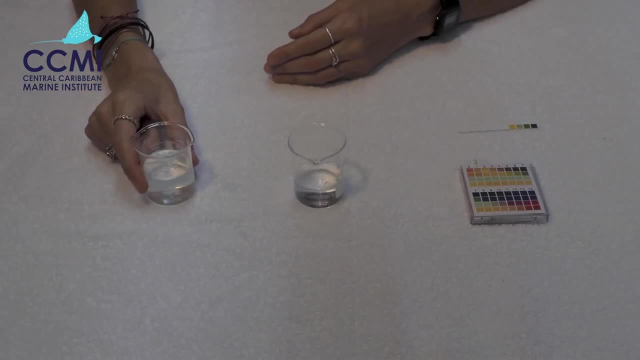 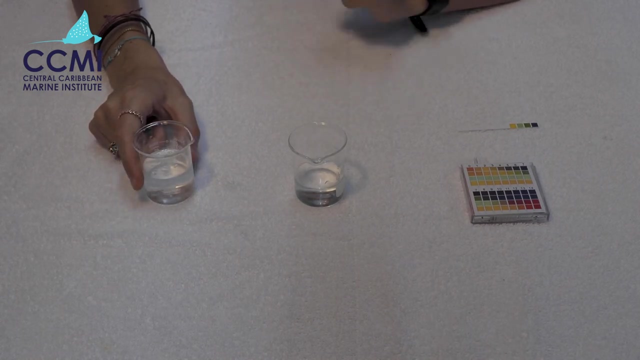 to mimic ocean acidification. now, inside this beaker that i have right here, i have just put in normal household white vinegar, which is readily available, and all i'm going to do is pour a little bit into this solution. here i'm going to take my wooden stick and i am going to 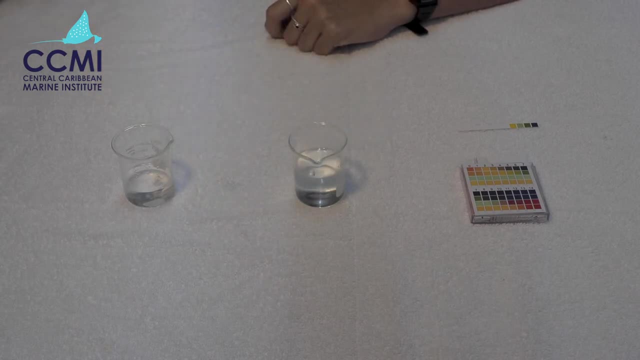 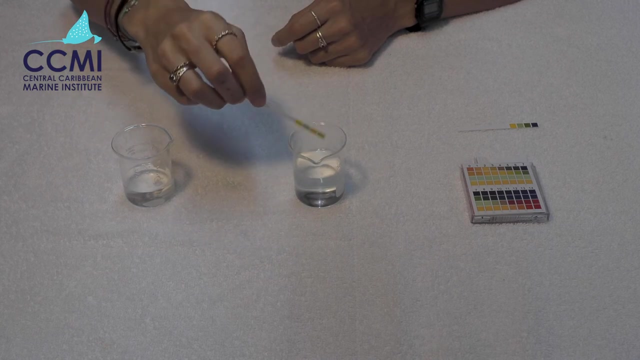 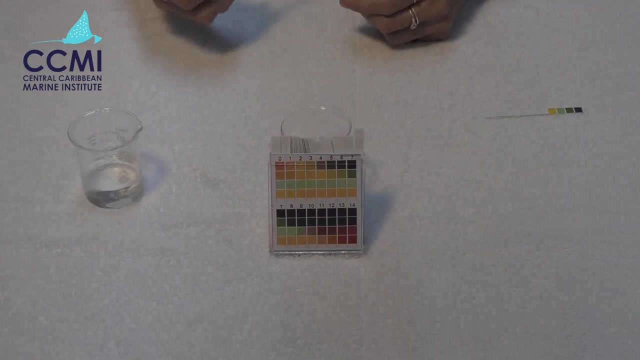 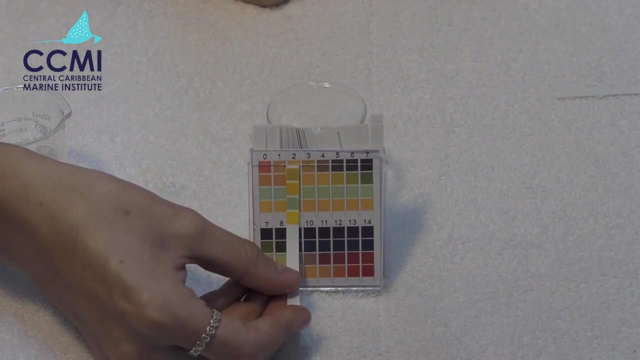 wrap it around. now. what i'm going to do is i am going to once again take my ph test strip. i'm going to dip it into the solution, take it out and then, coming back to our color code on the back of the packet, i am going to come over here and i'm going to say that this matches a ph of three. so we 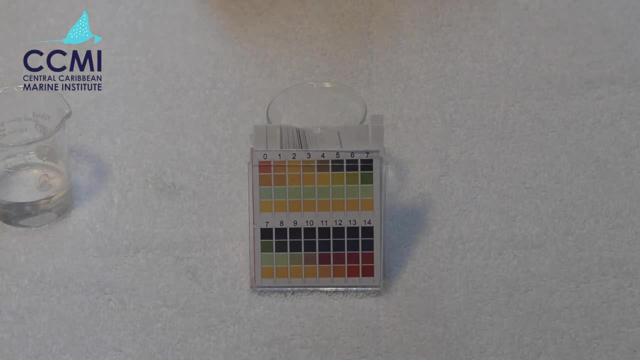 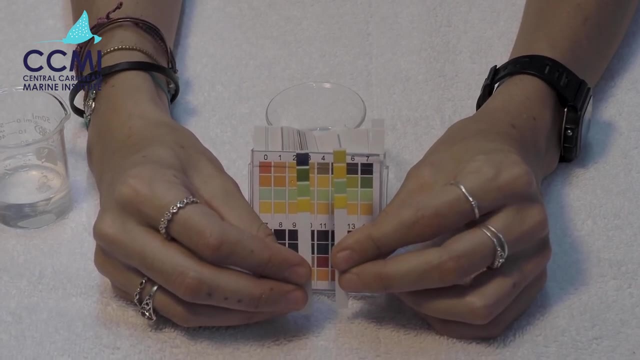 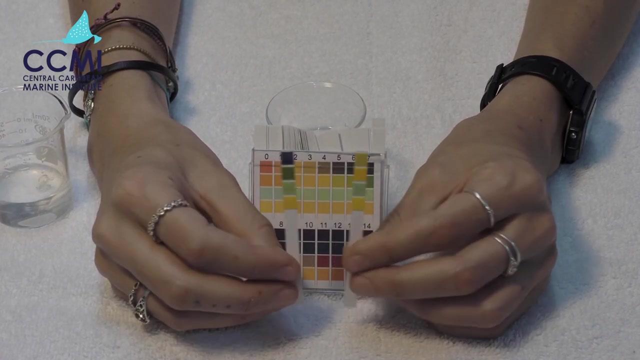 are going to take the ph from eight to three and if i hold these two test strips here, we can see how much the test strips have changed and how that is indicating the reduction in the ph between these two solutions. so that is the very simple experiment that we have provided. 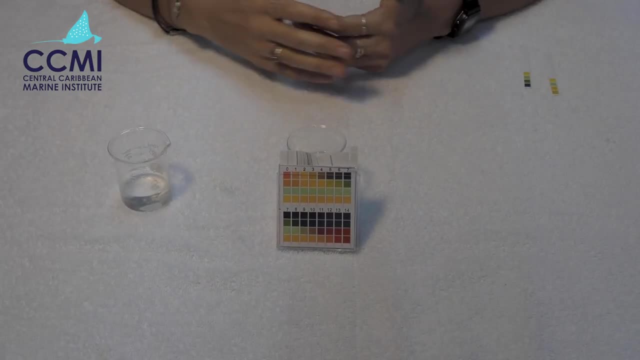 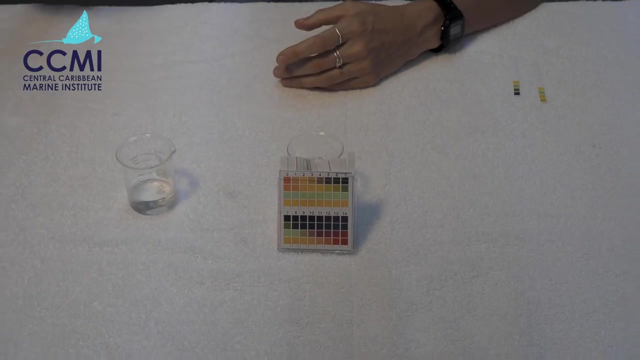 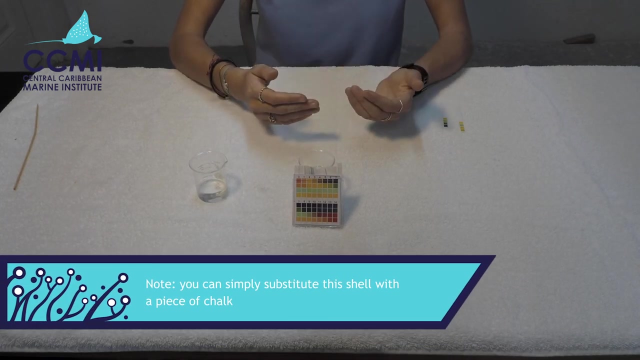 you guys the equipment for now. of course, you are more than welcome to expand upon this, and an experiment that you could easily undertake is: you could go to the shore and you could collect several very small shells from the shore. you could weigh them and then you could put one in a fresh. 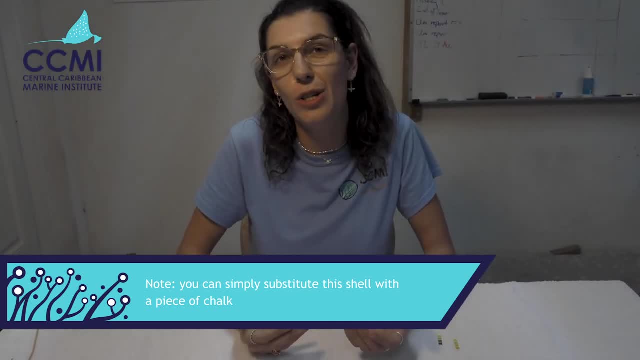 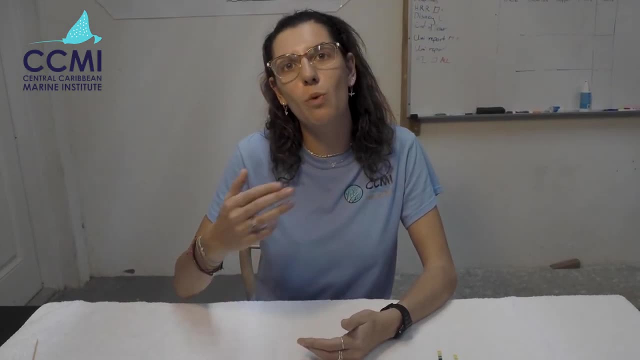 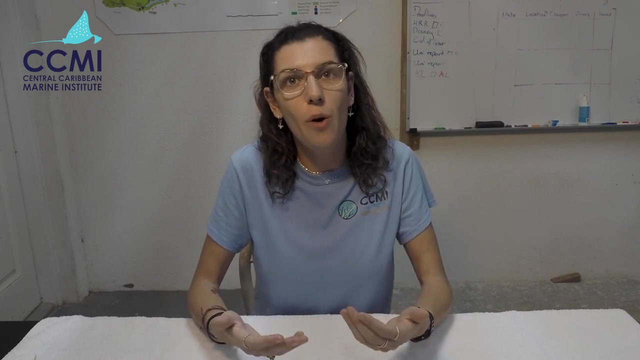 water solution and you could put, or a salt water solution and you could put one in a more acidic solution. leave them for a week and then you can go and weigh them afterwards as well, and what you're going to see is that the shell that was in the more acidic solution has actually degraded slightly.